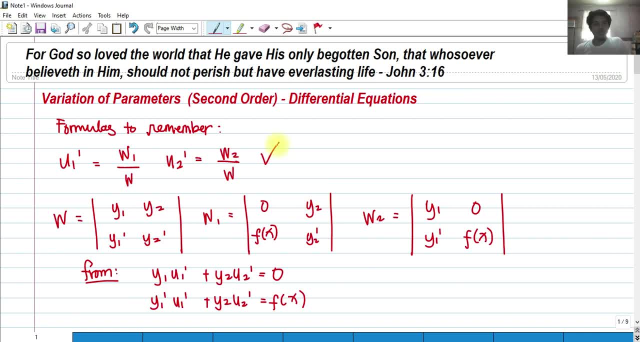 So this is basically Kramer's rule. This is only Kramer's rule. We have Ronskian sub 1 over the Ronskian and we have Ronskian sub 2 over the Ronskian. So remember, in our matrix, if we are getting the unknowns of the, for example, two equations, two unknowns, 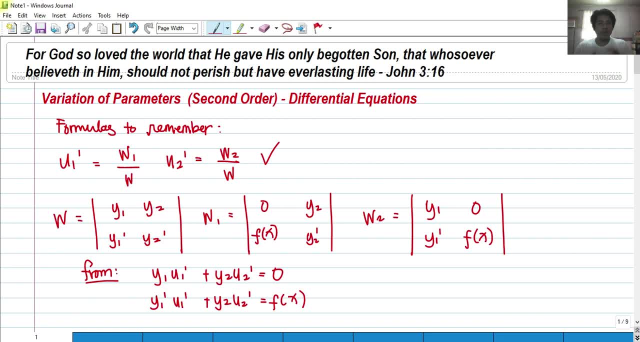 and we're going to get the unknowns by Kramer's rule. we may recall that we are simply replacing: okay, for example, in our Ronskian, these are the constants In Ronskian 1, we are going to replace the first okay, the first column by the constant. 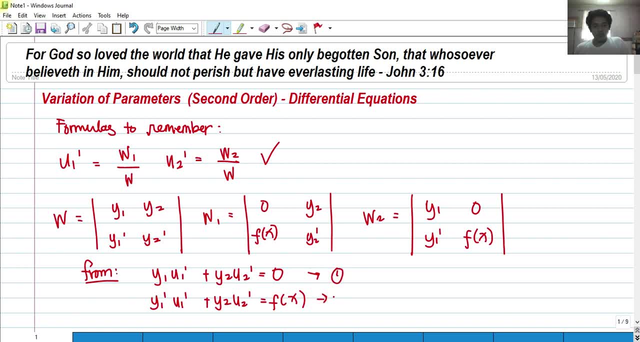 So you can imagine that this is our first equation in our second equation: okay, So we are going to replace. We are going to replace the constant okay, 0 and f of x, in this case okay, in the first column of w, sub 1.. 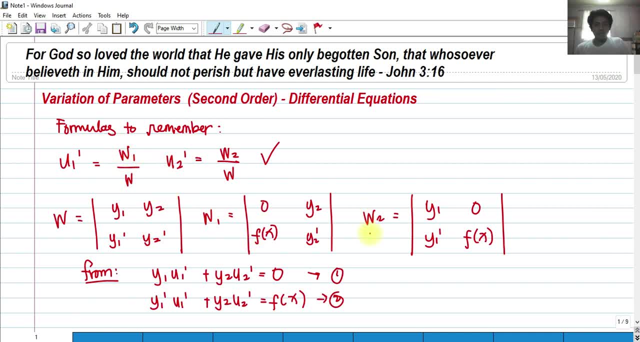 And get the determinant: okay, that's w sub 1.. And for w sub 2, you're going to copy the y sub 1 and y prime sub 1, okay, y sub 1, prime, okay, and then replace the second column by the constants, of which this is 0 and f of x. 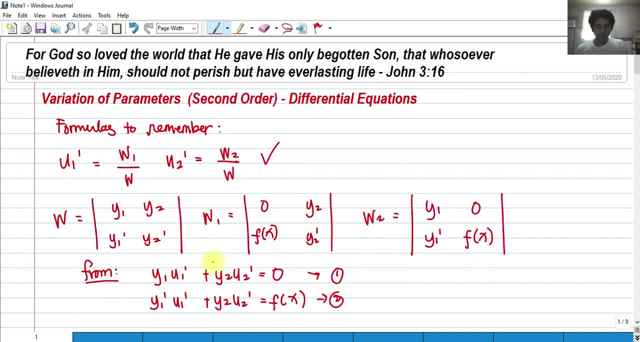 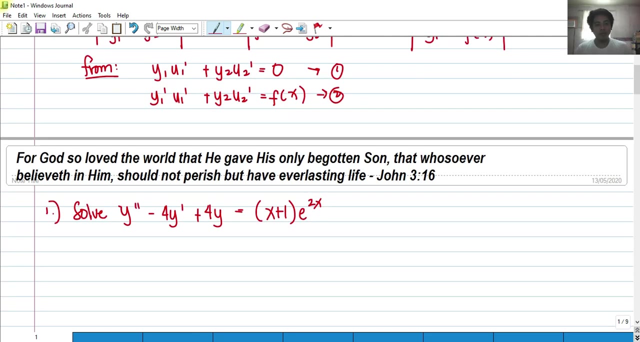 Actually, this is where we get our formula. Okay, It takes time, but as we go on to solve some problems, okay you will understand deeper what that or appreciate more this formula. So let's get started. I will show you how to solve a second-order differential equation by variation of parameters, step by step. okay. 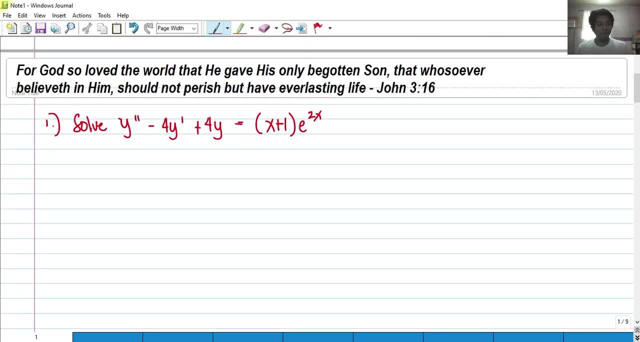 So we're going to solve this. solve y double prime minus 4y. prime plus 4y is equal to. We're going to write: the first thing that we're going to do here is to write the auxiliary equation. okay, Write the auxiliary equation. auxiliary equation. 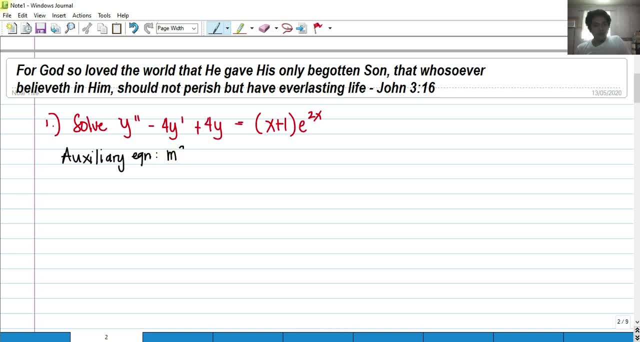 Okay, We know that we can replace this by m squared, because it's a second derivative, and then we have minus 4m plus 4.. equal zero. okay, remember that, whatever it is on the right side. okay, this is our f of x. this is: 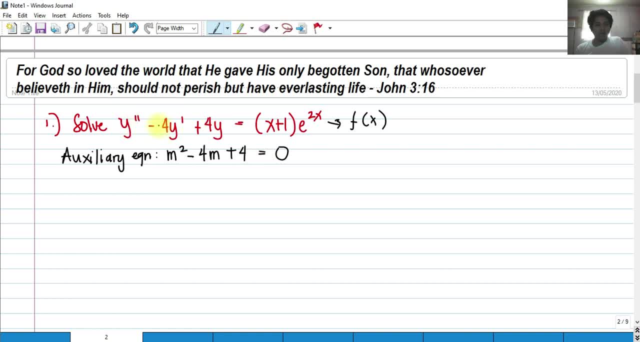 considered as constant. okay, because we have a dependent variable of y and it is this. one is all in terms of x, so this is constant, okay. so we have f of x. that is our f of x. so for our auxiliary equation, we're going to get the roots okay, and we know that that is equal to m minus 2. 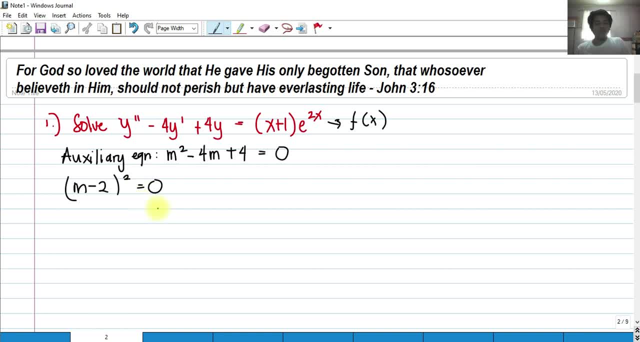 squared equals zero. so we have a root m sub 1 and m sub 2, which are both equal to 2. okay, then we have m sub 2, so this is a repeating root. okay, if you haven't watched my discussion. okay about auxiliary equation with repeating roots. 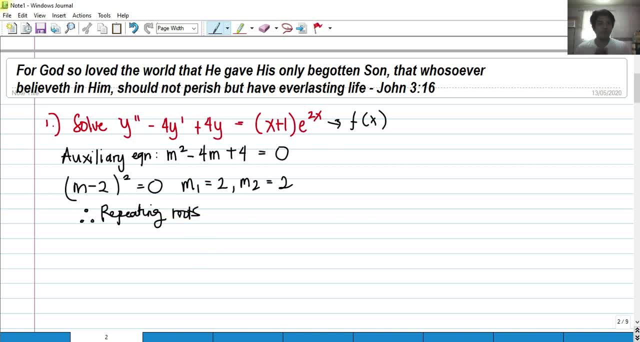 minus. well, first, uh, watch that before proceeding with this video, because it's actually we're going to apply what we have learned on that video. so it is a repeating root. so therefore its characteristic equation, or y sub c, can be now rewritten as, since it is repeating, we have c sub 1. okay, we have. 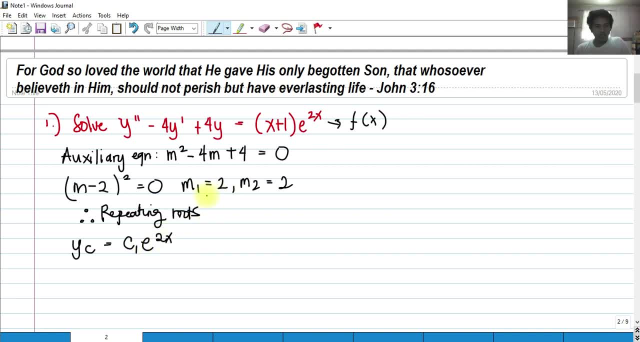 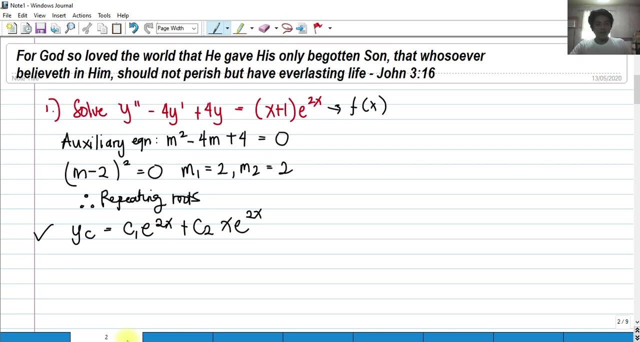 e raised to m sub 1, x, okay, which is 2 plus c sub 2. and then we have x, because it's repeating e raised to m sub 2 x. so this is now our characteristic equation, okay, so from here. from here, we can get y sub 1 and 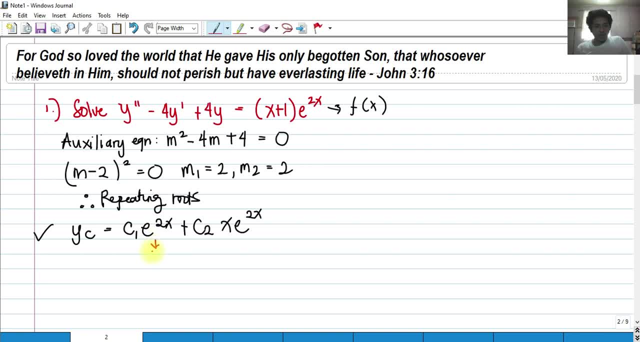 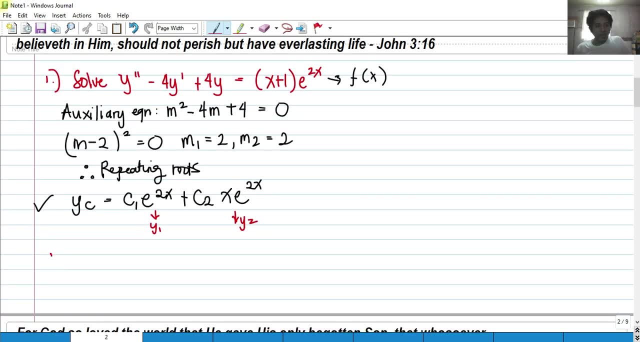 y sub 2. okay, in this case, this would be our y sub 1. this would be our y sub 2. so what we're going to do next is to get the ron scan. okay, first the ron scan, again, in order for us to get the ron scan. 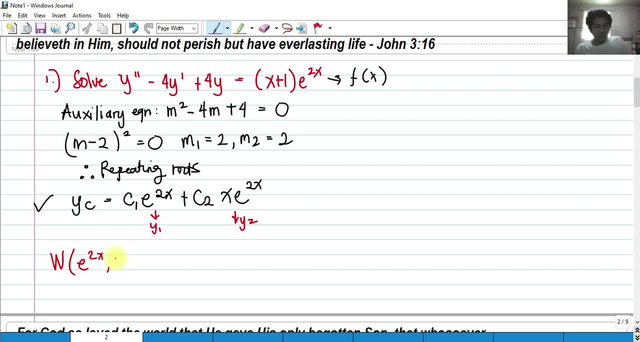 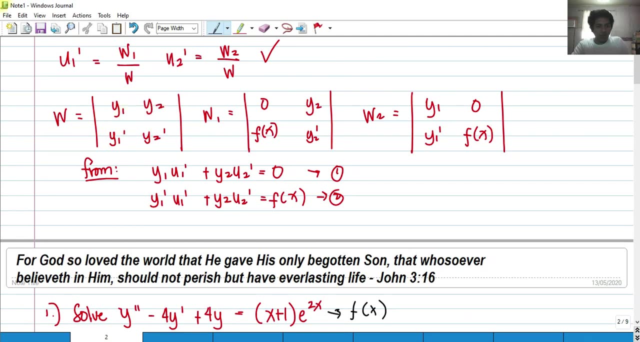 okay, we can rewrite it as e raised to 2x and x e raised to 2x. the ron scan of that is actually the determinant. okay, the determinant of y sub 1 and y sub 2 from our formula. okay, this is that: y sub 1. 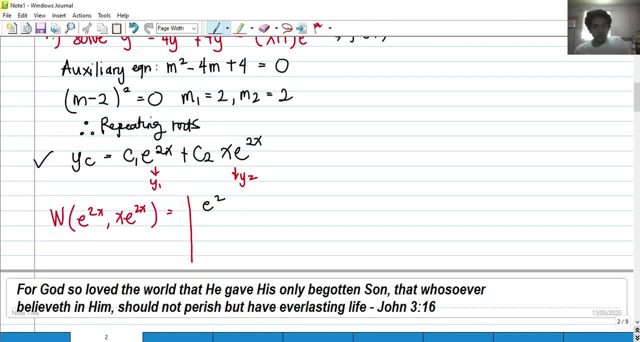 and y sub 2. so we have e raised to 2x, then we have x e raised to 2x, and then the second row would be composed of the uh uh derivative of each of these elements. so we have the derivative of this 2e raised to 2x. 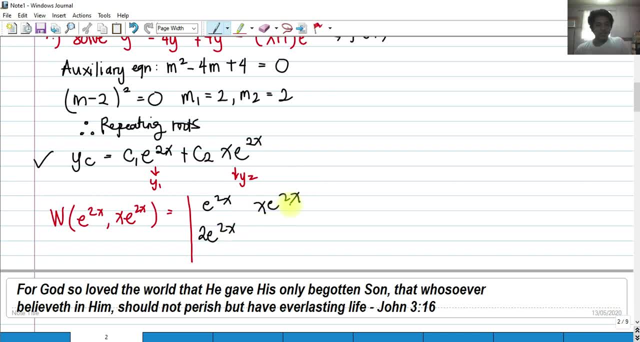 then if we differentiate this, this is actually what this is: product rule. so we have 2x e raised to 2x plus e raised to 2x and then we enclose that by our determinant okay. so in getting the determinant again, we need to get the product okay of this diagonal, minus the product of this. 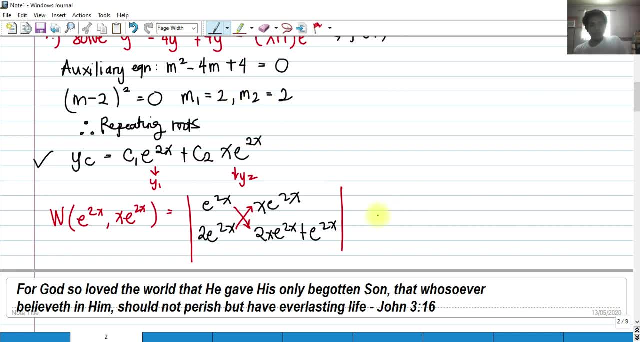 diagonal. okay, so first we get e raised to 2x multiplied by 2x, e raised to 2x plus, e raised to 2x minus the product of this two diagonal. so we have x e raised to 2x multiplied by 2 e raised. 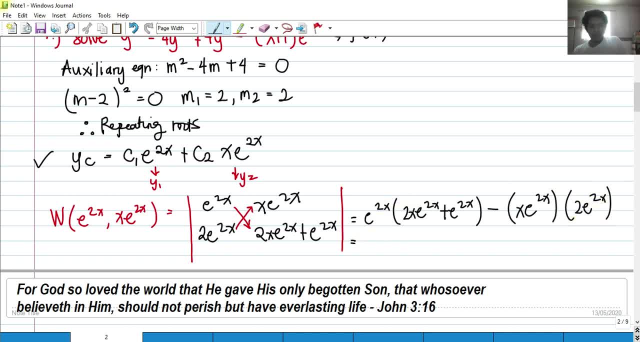 to 2x. so so if we evaluate that that would be 2x, okay, it becomes e raised to this become 2x. e raised to 4x, plus e raised to 4x. okay, if we multiply this, their, their exponents, add okay. so we have minus 2 e raised to 2x times this 2x e raised to 4x. so as you can see, 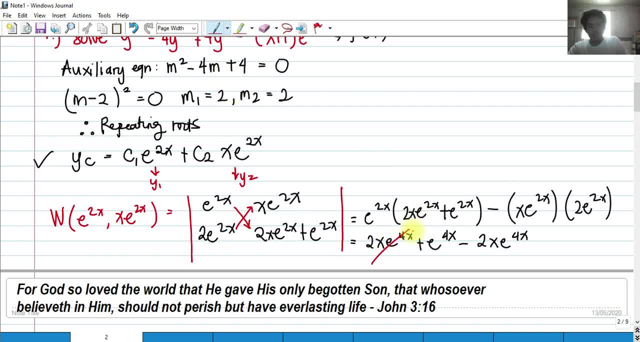 we can cancel, okay out this and this. hence we have an answer of e raised to 4x. it's a matter of the loss of exponent. that's why it became 4x. okay, so we add the exponents. okay, so that's the ronskian w. okay, so again we need to find. let me just uh. 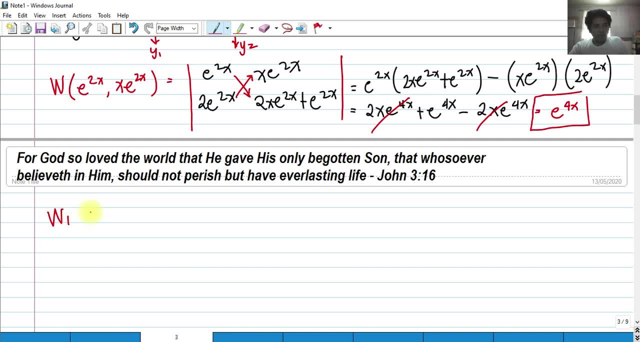 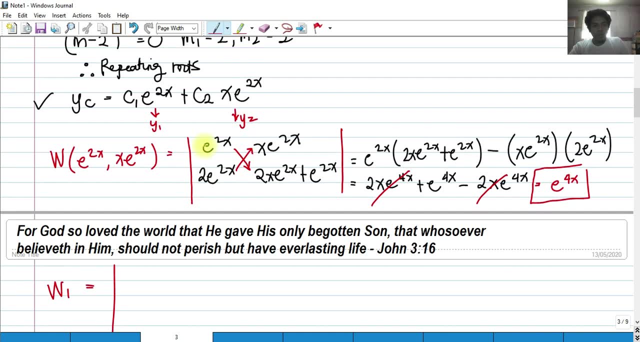 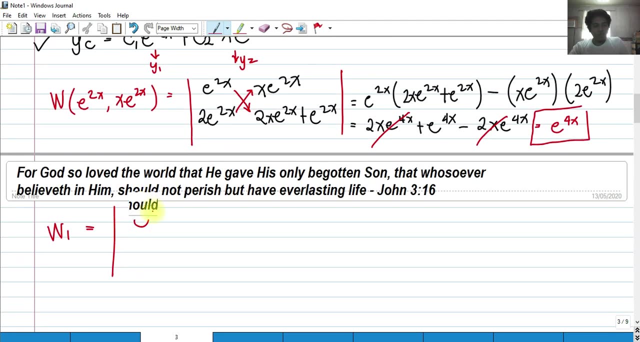 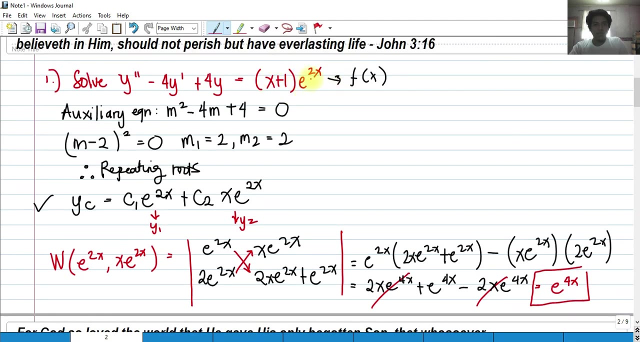 again rewrite w sub 1. what is w sub 1? we're going to replace the first column, this column, by the constants. okay, and we know that the first constant is 0, based from our equation on the formula, and the second one is the given f of X from our 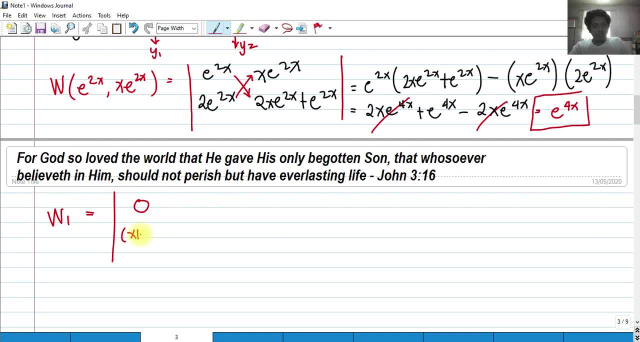 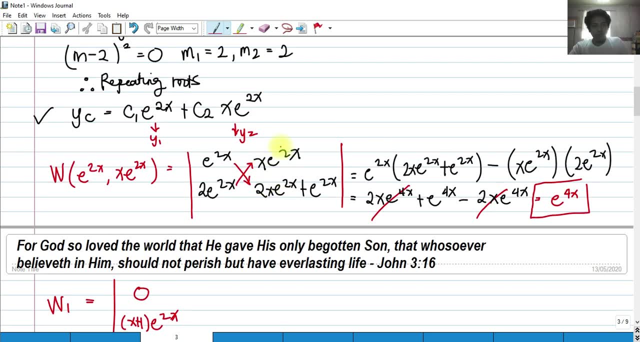 example. so we have X plus 1 e raised to 2 X. okay, and then copy the same column, second column of our Violet Rến Scкого: 1 Rånskian- original Rånskian. so we have x, e to 2x. 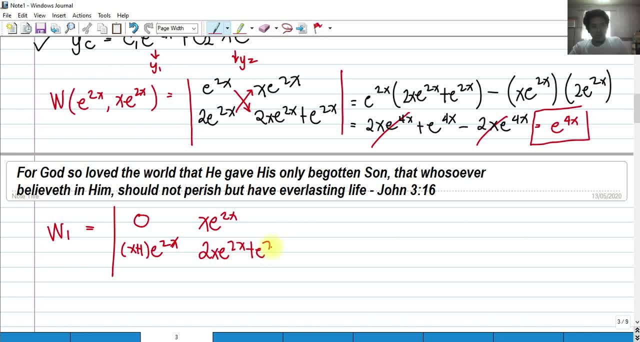 then 2 x e to 2 x, plus 6 e raised to 2x, then get the determinant, that's the Rånskian W1. okay, so we know that this is 0. okay, that's 0 minus. this diagonal is 0, then minus the product of. 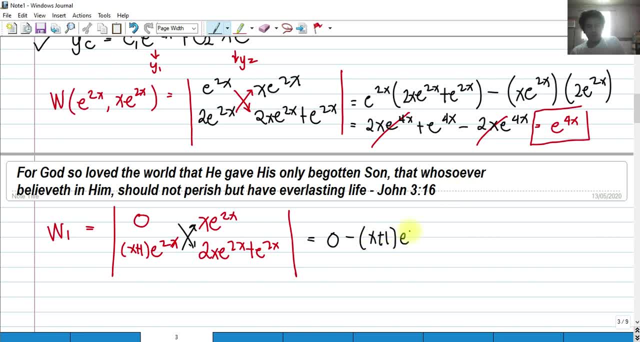 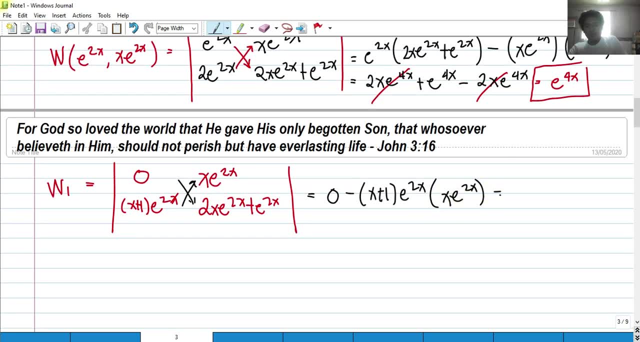 this. so we have x plus 1 e to 2 x, multiplied by x e to 2 x. so there we have it. So if we are going to simplify this, that should be negative x plus 1, then we have x e raised to 4x, okay. 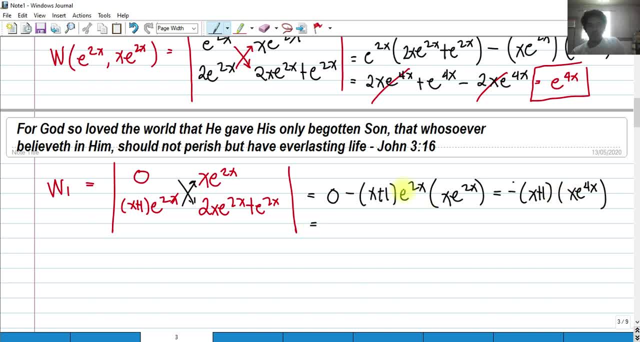 And then we simply multiply that, so we have negative x squared e raised to 4x, plus x e raised to 4x. okay, Okay. and again distribute the negative sign: negative x squared e raised to 4x, minus x e raised to 4x. then factor out some of the what do you call this? factors. 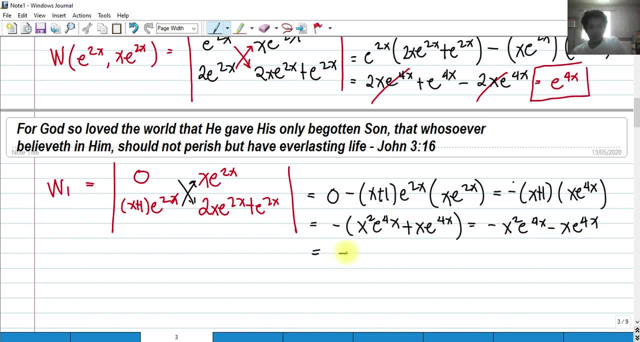 So e raised to 4x is both common as well as the negative. we can factor it out, so I can. we have x, okay, plus 1.. Okay, Okay, Okay, Okay, Okay, Okay, We have e raised to 4x. okay, that x, I mean we have x. e raised to 4x because we can factor both x here. x e raised to 4x. 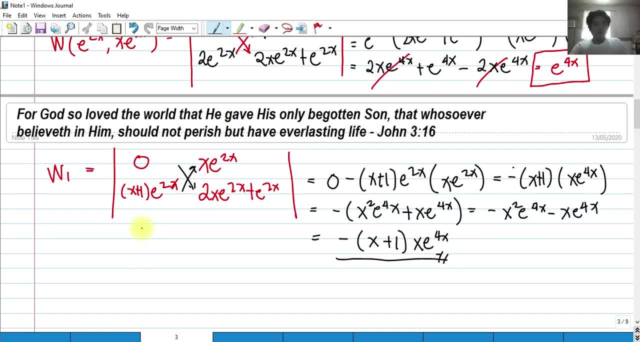 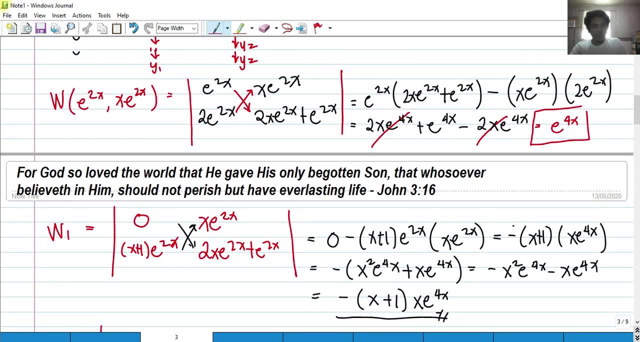 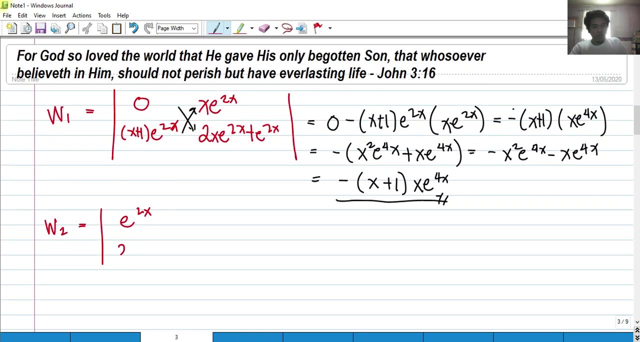 So that's our w sub 1.. How about for w sub 2,, okay, Ronskian, sub 2,. that is, we simply copy the first column, okay, of the original Ronskian. so we have e raised to 2x, all over 2. e raised to 2x for our. 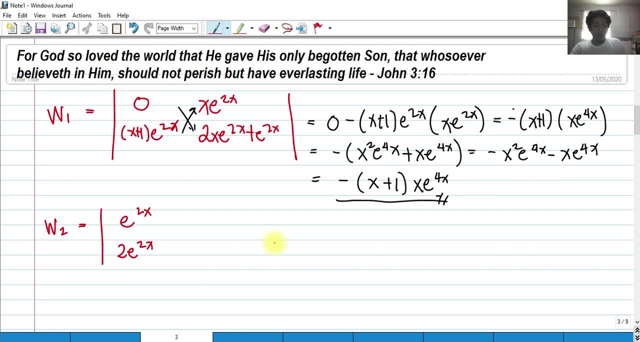 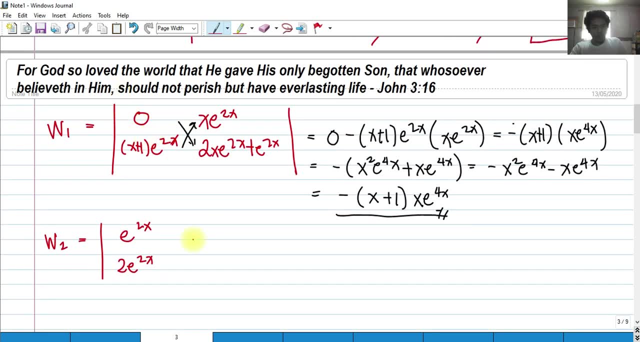 second row, second column, our first column, second row, and then we have- we're going to replace the second column by the constant, so we have 0 and f of x, which is x plus 1 e raised to 2x, and get the determinant of that. 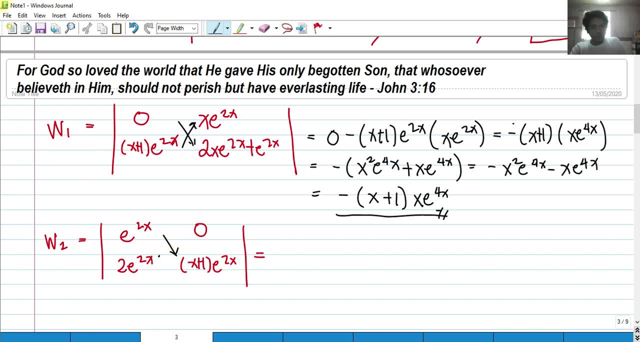 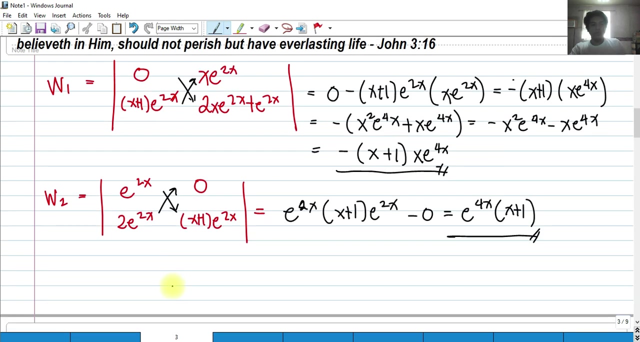 So, upon getting the determinant of that, we know that this is minus 0,. okay, this should be 0,. I'll rewrite that later on, Okay, Okay. So what will happen if we multiply this? this should be e raised to 2x, okay, and then multiplied by x plus 1, e raised to 2x minus 0, and that is e raised to 4x, x plus 1,. okay, that is our Ronskian sub 2, w sub 2.. 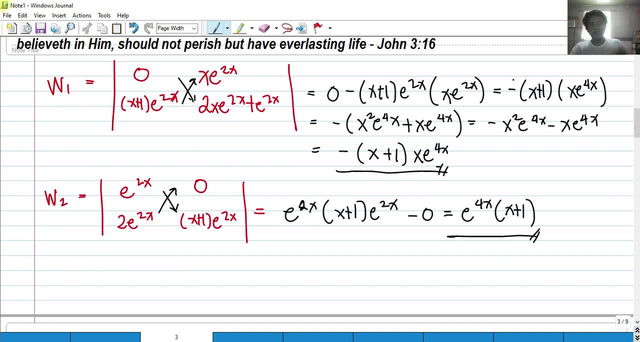 Now it is time for us to get the u sub 1 prime and the u sub 2 prime. So how do we get that Again from our formula u sub 1.. So we have the w sub 1 prime, that is, w sub 1 over w. 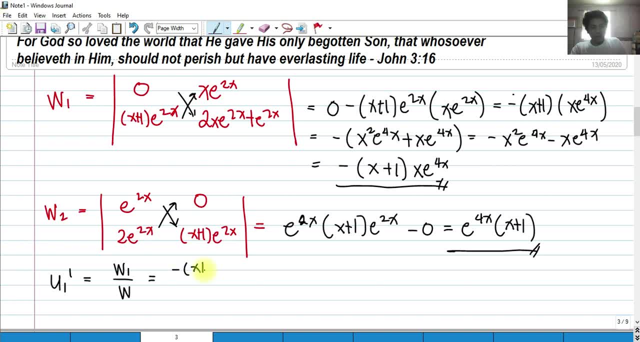 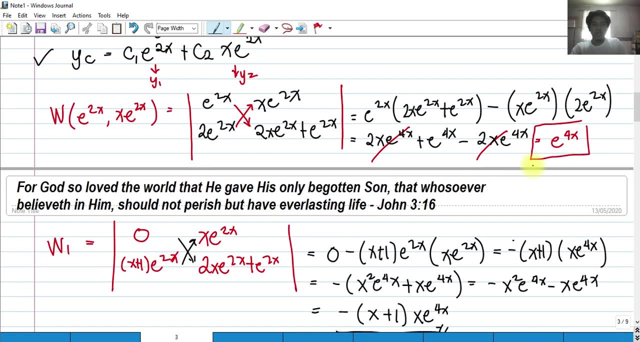 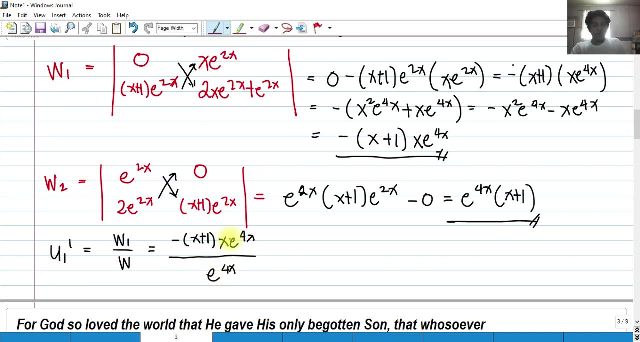 So we have the w sub 1 as this negative x plus 1 x, e raised to 4x, all over the w which is e raised to 4x, e raised to 4x. Since this is the numerator is multiplication, we can cancel it out. 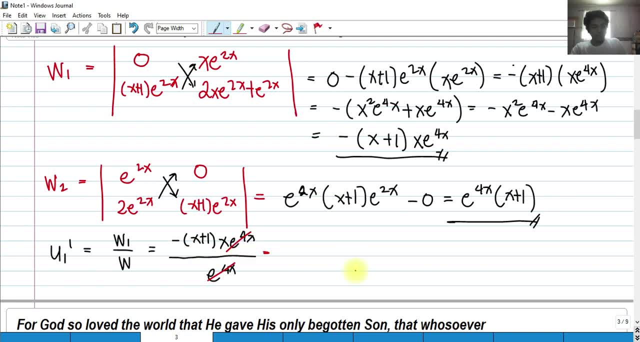 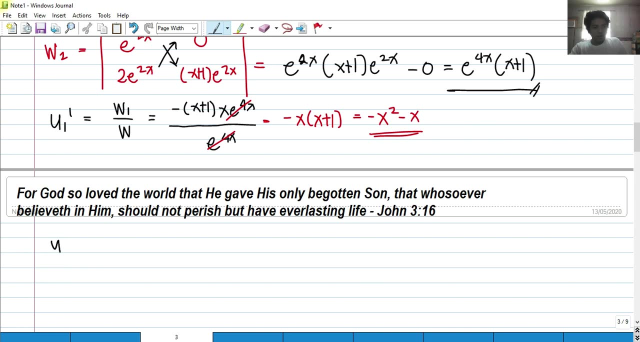 So we have the term. okay. So we have negative x times x plus 1, of which that is negative x squared minus x. okay, that is our u1 prime. u sub 1 prime. How about u sub 1, u sub 2 prime, okay? 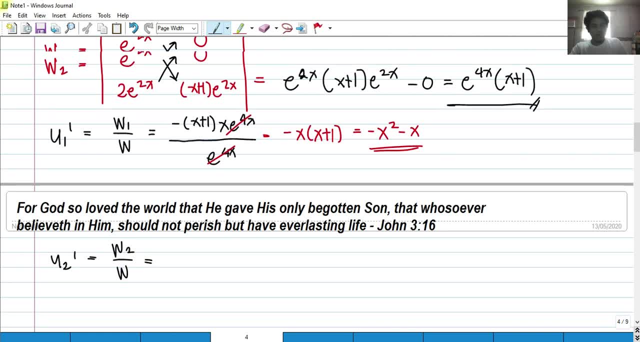 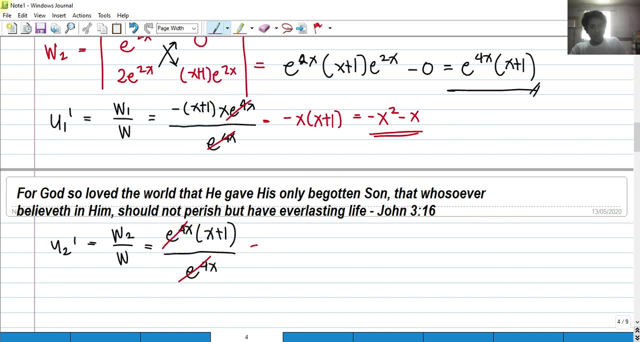 So we have w sub 2 over w, so w sub 2 is e raised to 4x. x plus 1 multiplied by x plus 1 all over our w is e raised to 4x. So definitely that would cancel leaving us x plus 1 for our u sub 1 prime and u sub 2 prime. okay. 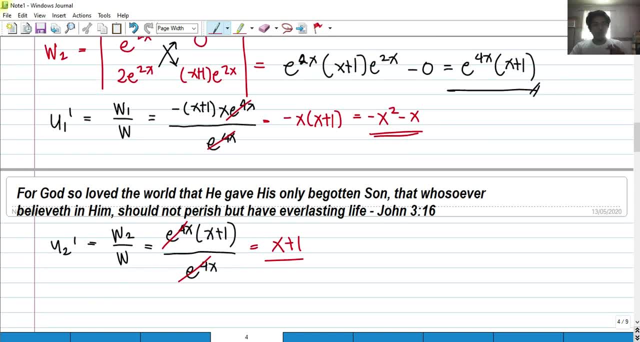 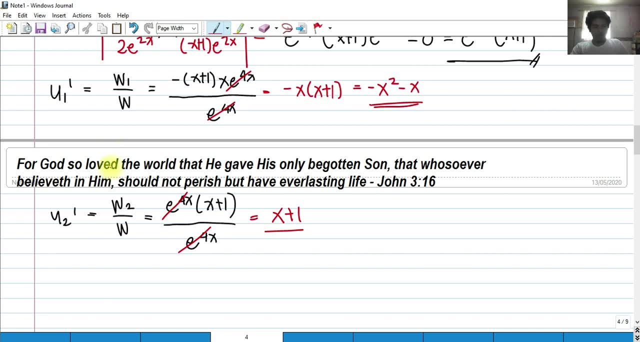 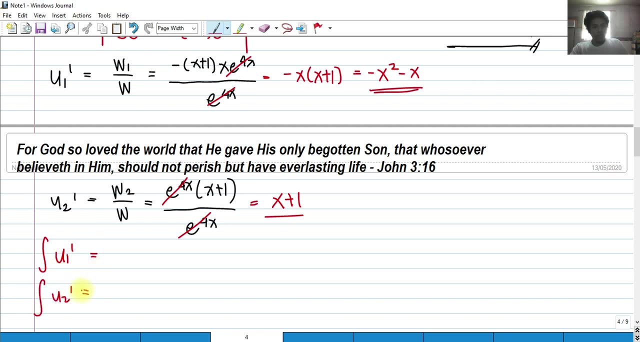 That is not the final answer. What are we going to do is to integrate u sub 1 prime and u sub 2 prime, so that it becomes u sub 1 and u sub 2.. So if we integrate, okay, u sub 1 prime and integrate u sub 2 prime, well, of course it is in terms of x. 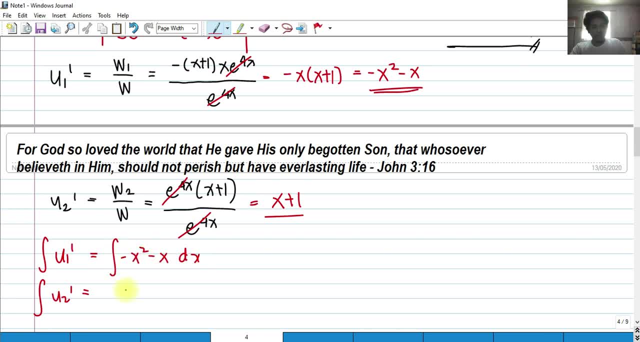 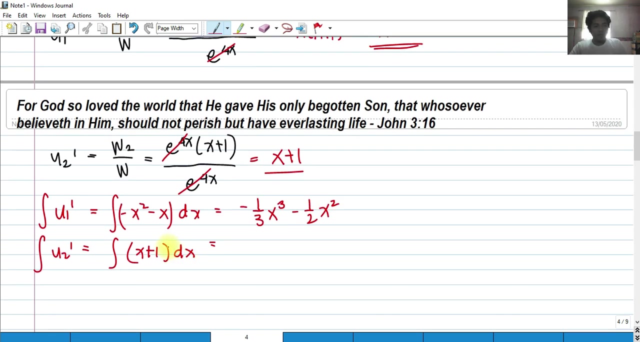 If we integrate that in terms of x, okay, in terms of x. so what will happen? we know the answer. it is very easy. It is just a power rule. power rule. so we have negative 1 third x cubed minus 1 half x squared. then we have x plus 1. here we have 1 half- okay- x squared. 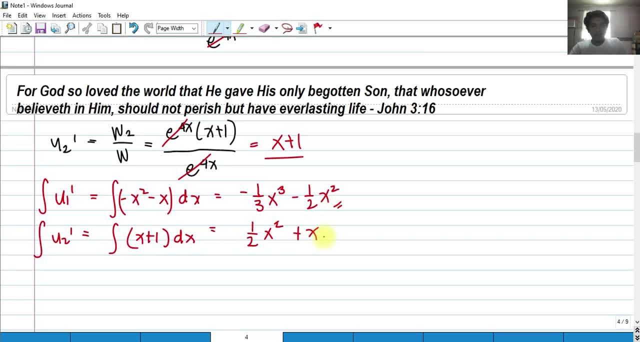 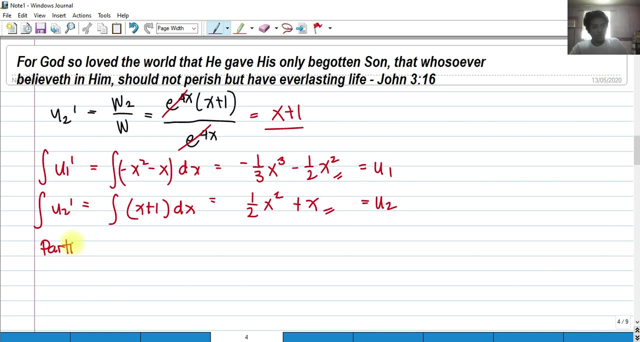 That is the integral of u sub 1 prime and u sub 2 prime. so this is now equal to u sub 1 and this is now equal to u sub 2.. Then what we're going to do next is to get the particular solution. particular solution. okay. 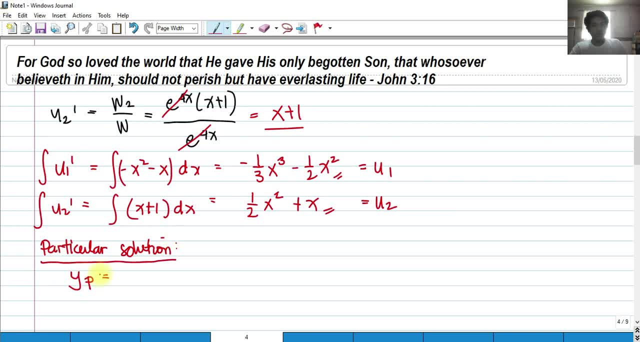 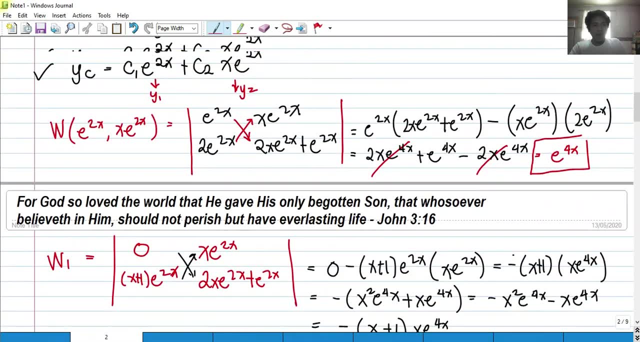 So we have particular solution. we're in, we're going to substitute, okay, Okay, Okay, Okay Okay, u sub 2. okay, in our characteristic equation c sub 1 plus c sub 2 as c sub 1 and c sub 2. 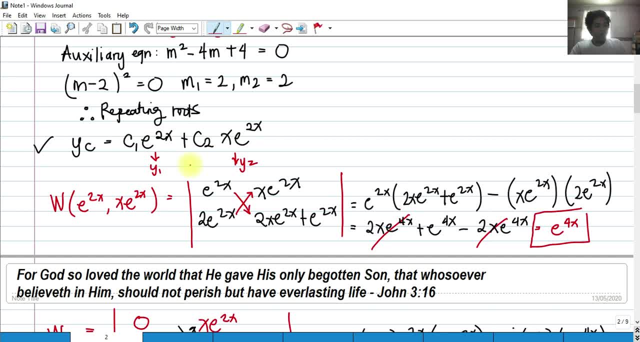 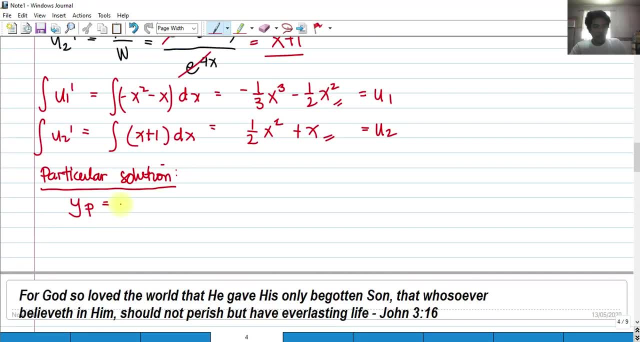 so this c sub 1 and c sub 2 will now be equal to that of we get u sub 1 and u sub 2. so what will happen? that is negative: one third x cube minus one half x squared. this is the c sub 1 and this. 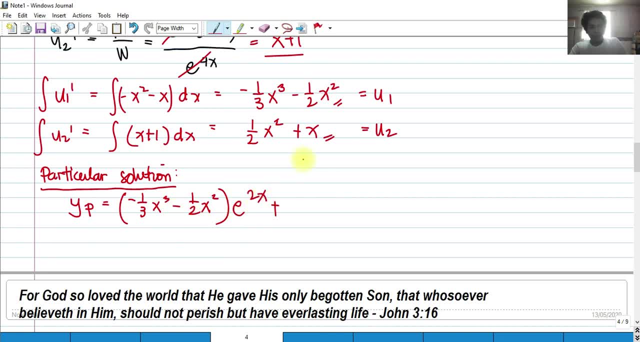 is multiplied by e raised to 2x, then plus c sub 2, this is our c sub 2, u sub 2. we have one half x squared plus x, and then we have x, e raised to 2x. now we're going to simplify this and upon 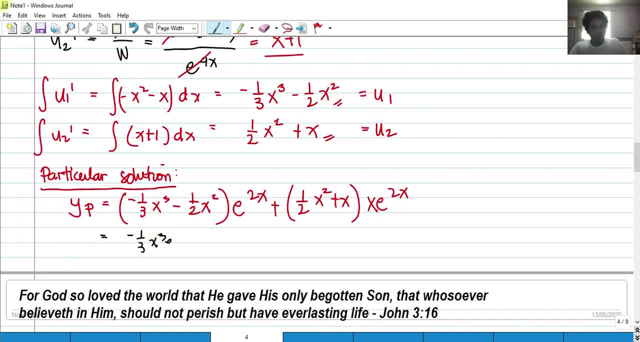 simplifying this. we have negative one third x cube e raised to 2x, minus one half x squared e raised to 2x, plus one half x you cube e raised to 2x. just, uh, distribute plus x squared e raised to 2x. so, as you can see, we can. 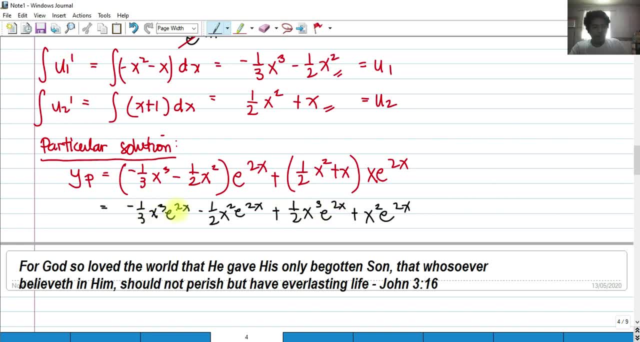 simplify: one half x cubed e raised to 2x and negative one half, uh one third x cubed e raised to 2x and that is equivalent to one sixth x cubed e raised to 2x and, as you can see, also negative. 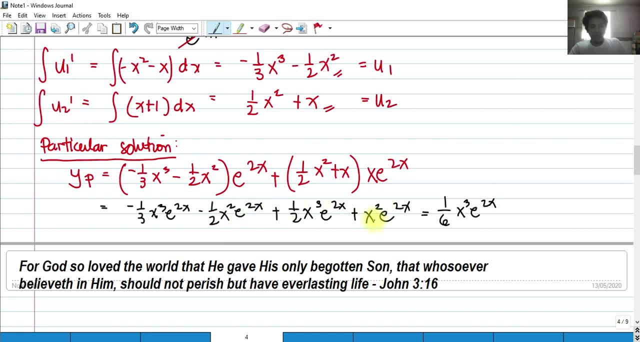 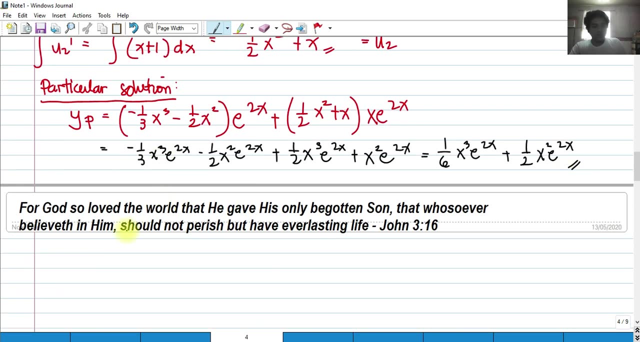 one half x squared e raised to 2x, and x squared e raised to 2x can now be simplified as: plus one half x squared e raised to 2x. okay, so, hence, this is our result for the particular solution. hence, therefore, our y or the solution to our second order differential equation. 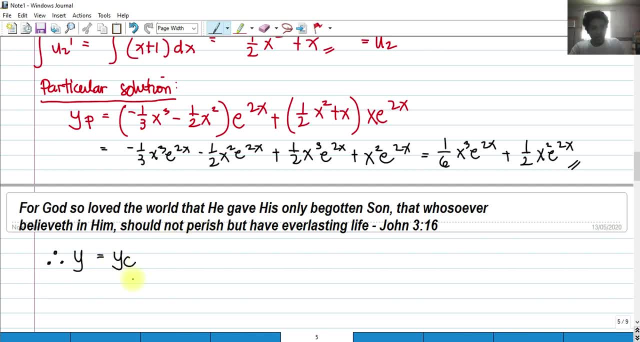 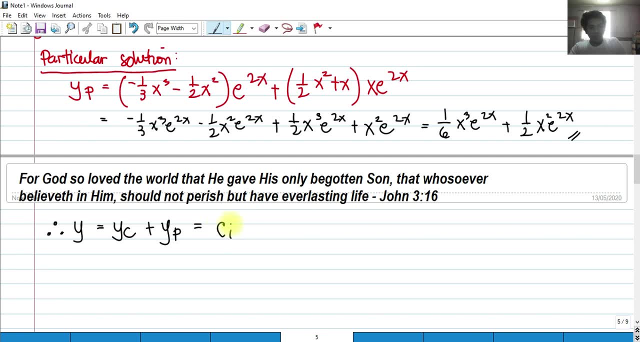 is the combination of y sub c, the characteristic equation, plus the particular solution y sub p, wherein this should be the answer: c sub 1 e raised to 2x plus c sub 2 e. okay, c sub 2 x. i mean okay, c sub 2 x. c sub 2 x e raised to 2x plus 1, 6 x. cube e raised to 2x. 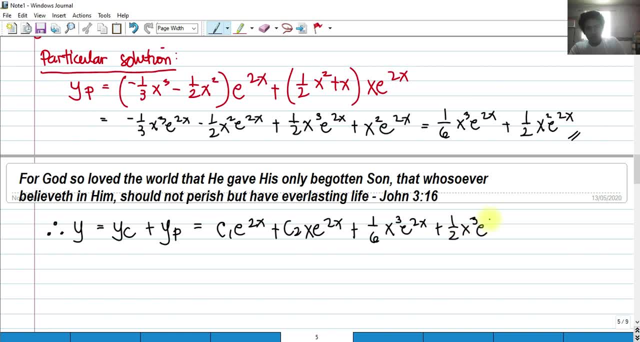 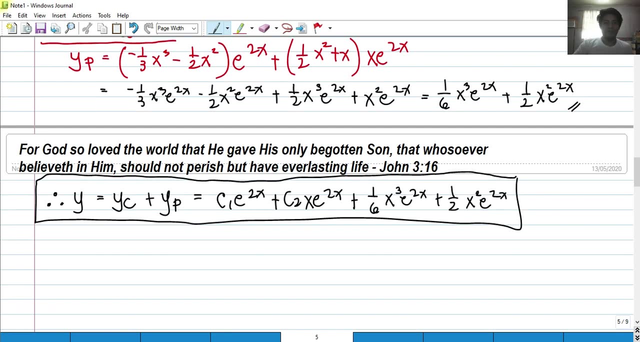 plus 1 half x cube or x squared, i mean that's x squared, x squared, e raised to 2x. so this is our answer for this particular problem. okay, i hope you understood, or understand, that process. so, in order for us to really practice more, okay. 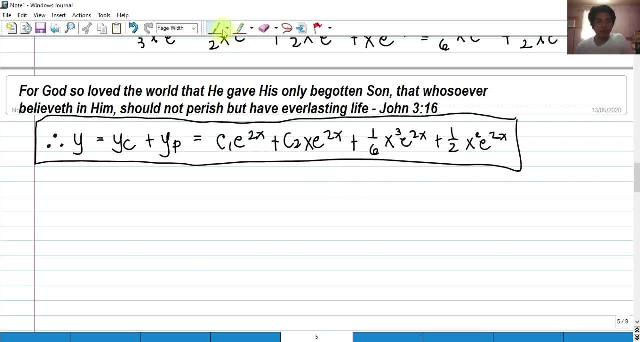 you need to solve another problem. this will be our last problem for this video. so for number two, we need to solve the Y double prime. for Y double prime, all right, plus 36 equals for second of 3x. so if you see a differential equation like: 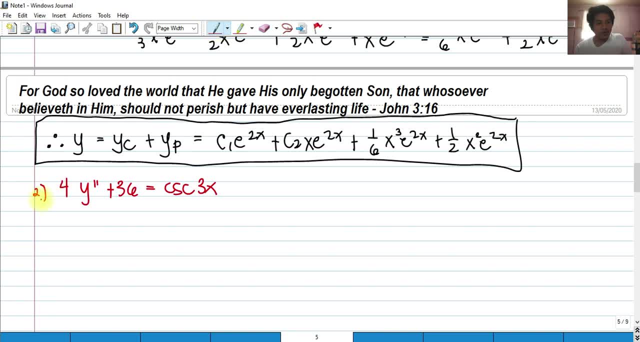 this: okay, so the highest order Y double prime has a constant greater than 1. okay, so it is good to put this into standard form. so what we need to do is to divide that both side of the equation by 4, so that we have Y double prime plus. 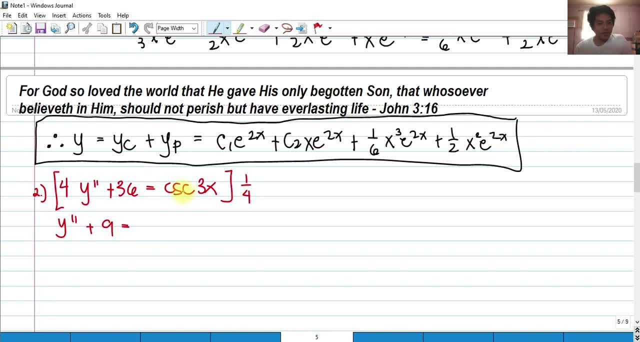 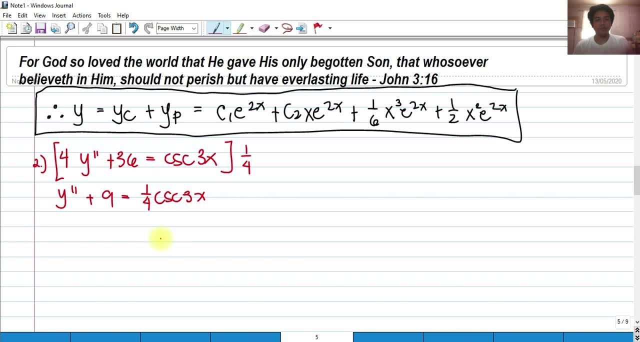 okay, we have 9 equals 1. 4th cosecant: 3x. okay. so, and again, repeating the process is still the same. the process is still the same. first, we need to get the auxiliary equation. so this is: M squared plus 9 equals 0, and we know that the roots of this is: 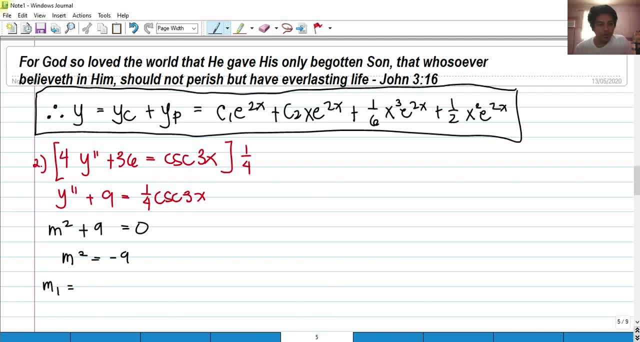 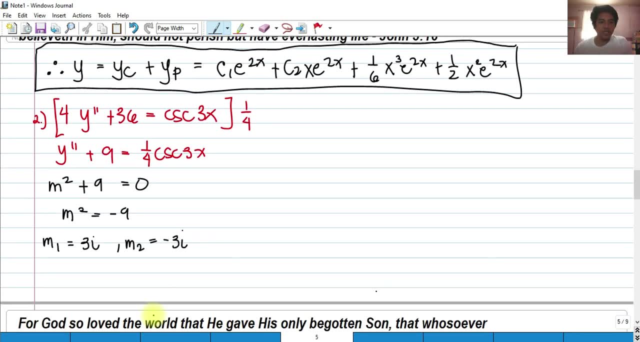 imaginary. so our M sub 1 would be 3I and our M sub 2, 2 would be negative 3I, and we write the auxiliary equations for the complex roots: alright, so our characteristic equation, I mean y sub z, would be c sub 1 cosine of 3x, plus c sub 2 sine of 3x. this is our characteristic equation. 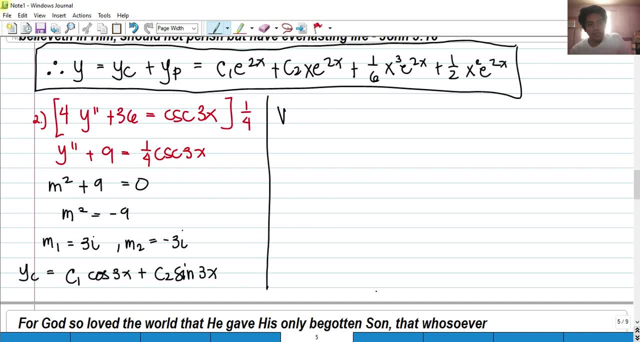 and again we need to get the ronskian. okay, so the ronskian would be cosine of 3x. this one, and the second row, second column, would be sine 3x and get the derivative of this. that is negative: 3 sine 3x. this is 3 cosine of 3x and get the determinant. so the determinant again is this: 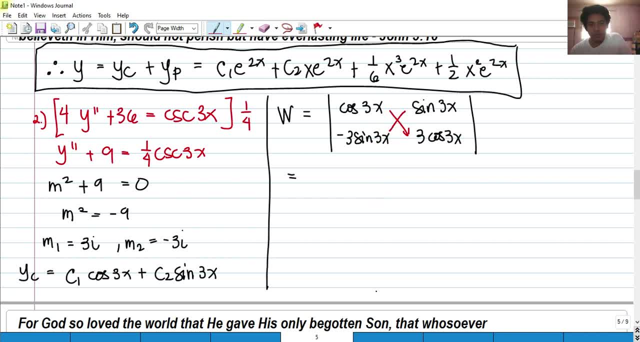 one, the product of this one minus the product of the other diagonal. so we have that would be 3 cosine squared 3x, because cosine 3x times cosine 3x is cosine squared 3x. then we have minus. okay, we have the minus and the product of this. please be careful with the minus sign that this this: 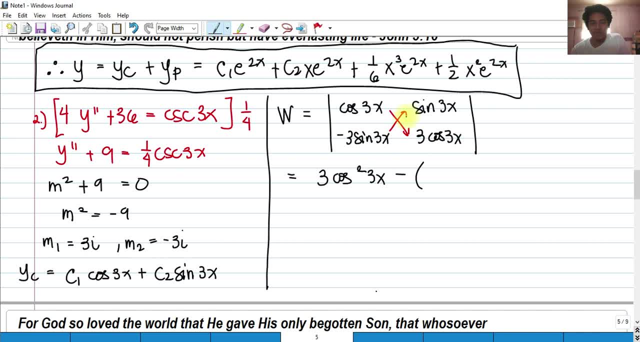 minus sign is not the negative one here, so we need to include still the negative here. so we have negative 3 sine squared 3x. then we have 3 cosine squared 3x plus 3 sine squared 3x. we can factor out 3 because that's common. we have cosine squared 3x plus sine squared 3x, and this is 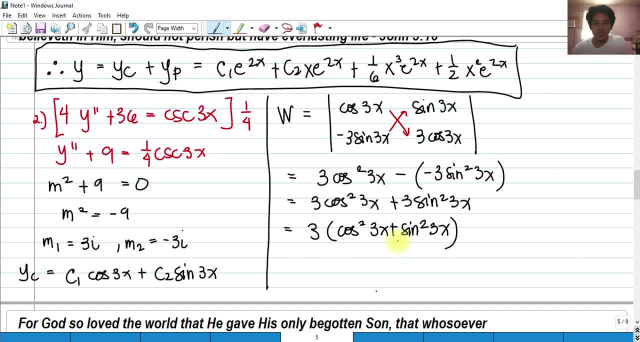 an identity where, if we have cosine squared theta plus sine squared theta, that is equal to 1, so we have 3 times 1. this is simply equal to 1, so we have 3 here. okay, the ronskian w is 3 again. the. 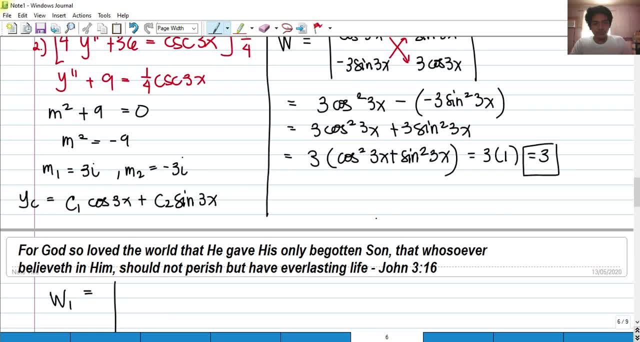 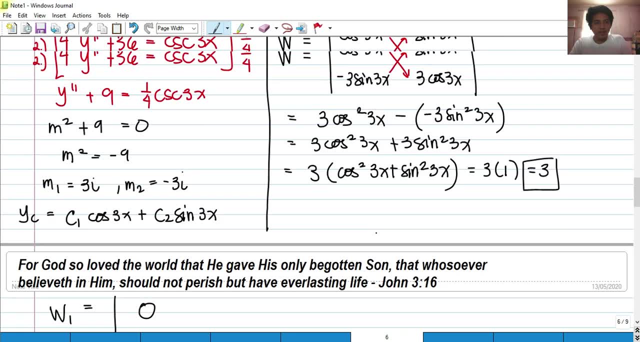 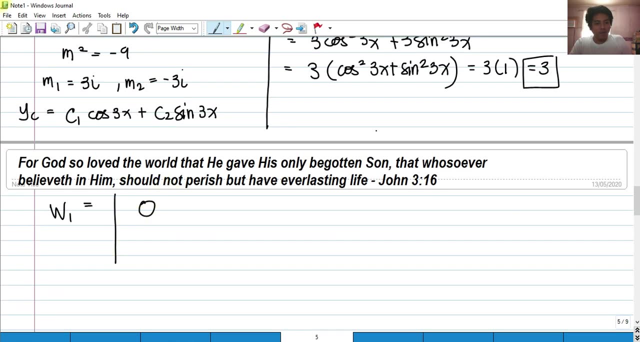 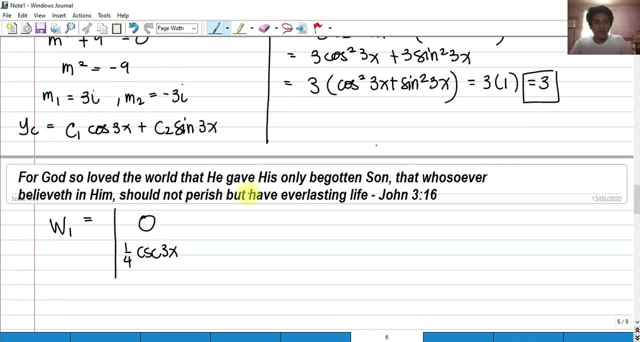 next one, w, sub 1. okay, we need to replace the first column- okay, by the constant, and the first constant is 0 and in this case, our f of x is this: okay, that is our f of x, so we have 1, 4 coseconst, and copy the second column, so the second. 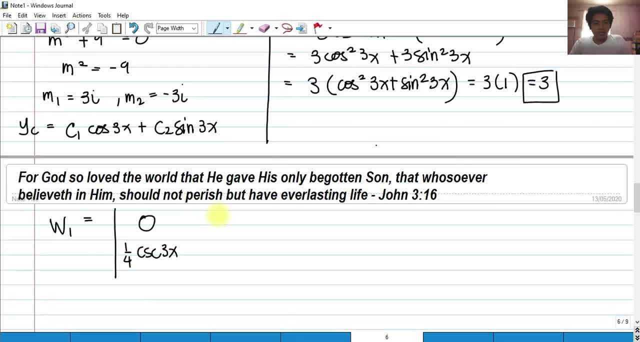 column is sine 3x, called 3 cosine 3x. so we have sine 3x, 3 cosine 3x, sine 3x cosine 3x, 4 cosine 3x. so that's how to make a frклад because very few of you of what we discussed class before will feel. 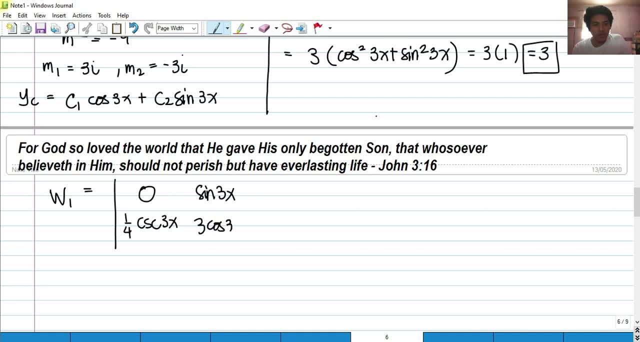 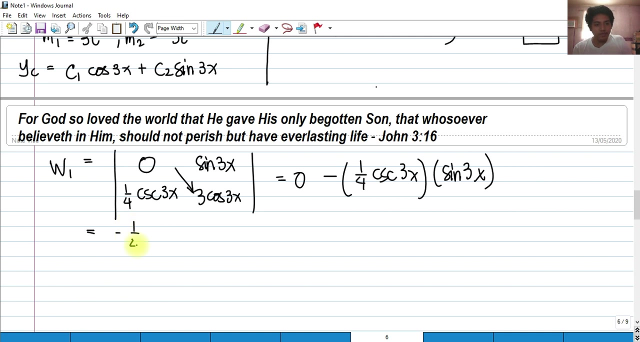 easy and nice when we want to kill your. We know that this would be 0, so that is 0 minus the product of this. so we have 1 fourth cosecant 3x multiplied by sine 3x. By using some identities, inverse identity- this negative 1 fourth cosecant is now equal to 1 over sine 3x and multiplied by the sine 3x. 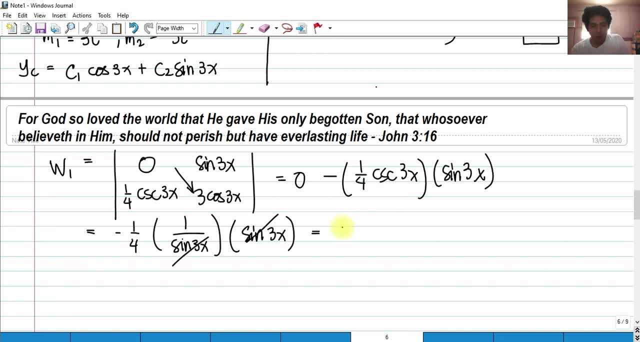 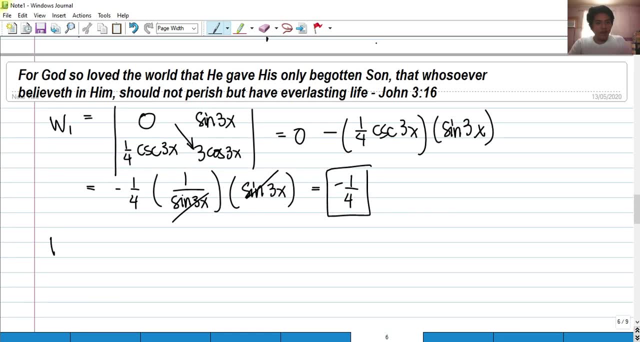 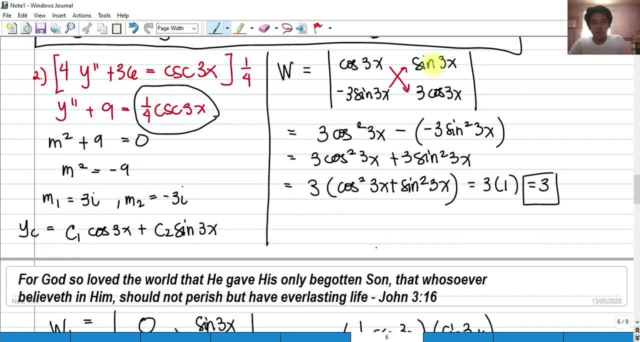 So, simply, this would cancel. so we have a W sub 1 or Ronskian as negative 1 over 4, or negative 1 fourth, Okay, And Finally, we have W sub 2, okay, as we are going to replace the second column, okay, by the constants. 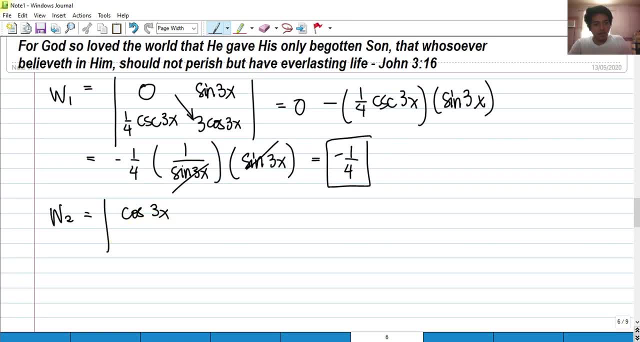 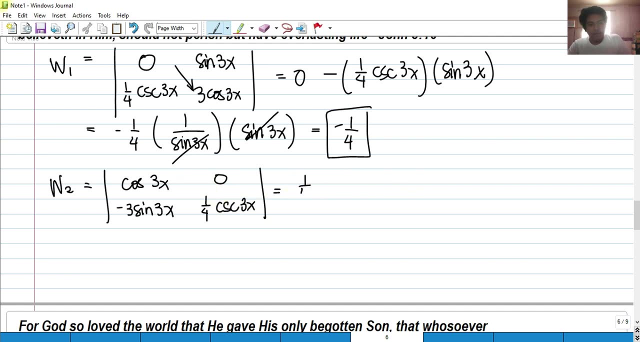 So we have cosine 3x and then we have negative 3 sine 3x, then we have 0, then we have 1 fourth cosecant 3x. Okay, So we have 1 fourth cosecant 3x. 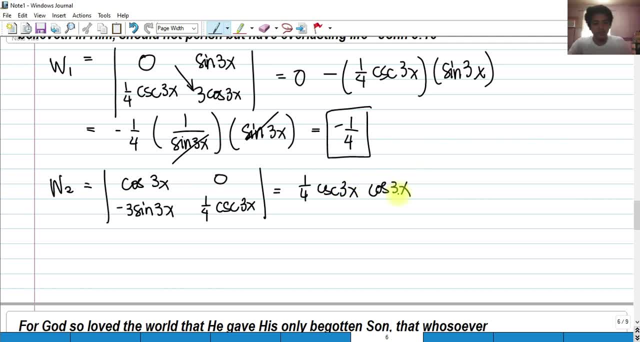 Multiplied. Multiplied by cosine 3x. Okay, So I would just use the identity here. That would become 1. fourth. So cosine 3x all over. That would become cosine 3x all over the sine of 3x. 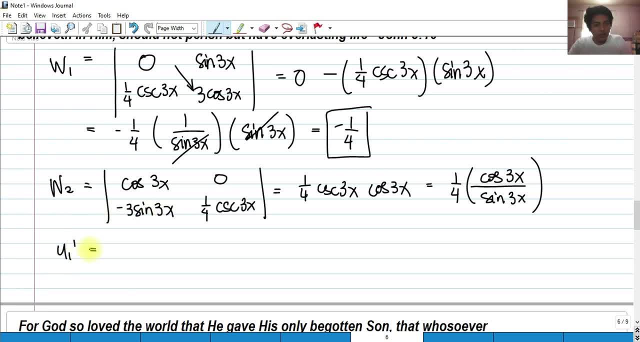 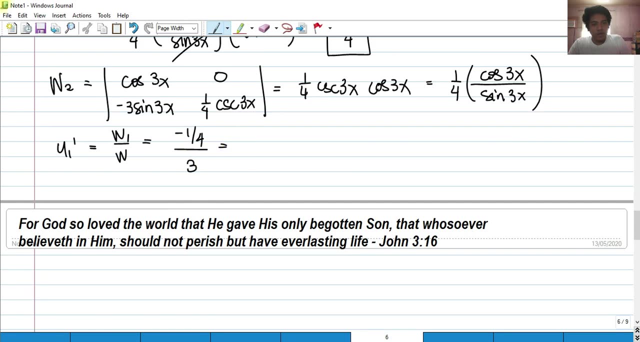 And get the U sub 1 prime, which is W sub 1 over W. W sub 1 is negative 1. fourth, all over W, Our W is 3.. Okay, So that would be negative 1 over 12.. That's our U sub 1 prime. 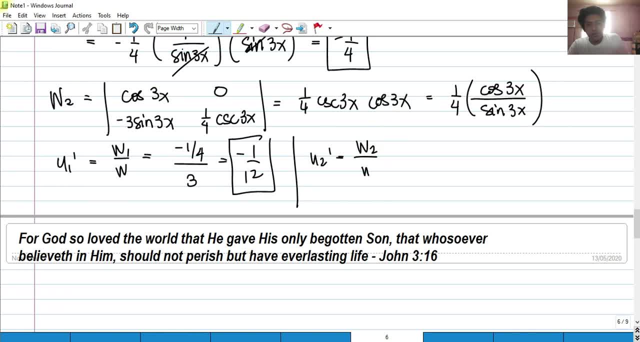 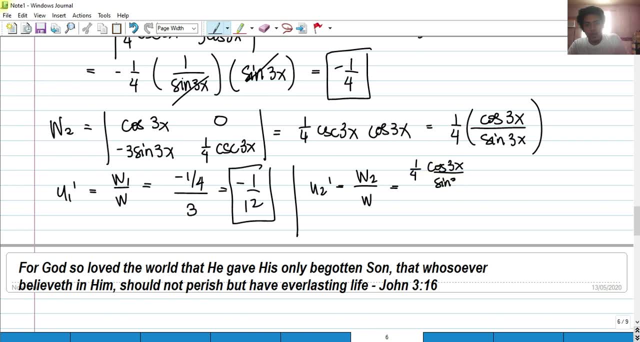 And then U sub 2, prime would be W sub 2 all over W. Okay, So we have 1 fourth cosine 3x all over sine 3x all over 3.. Okay, So what will happen? We have 1 over 12 of the cosine of 3x all over sine 3x. 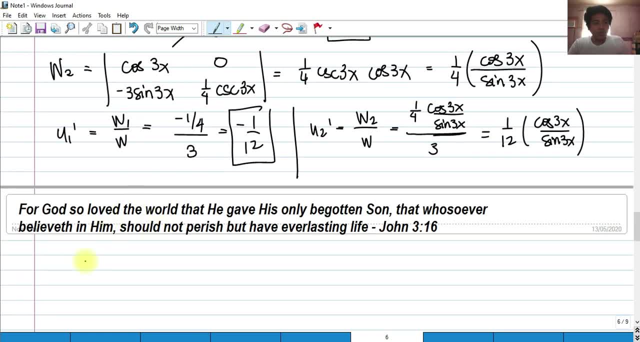 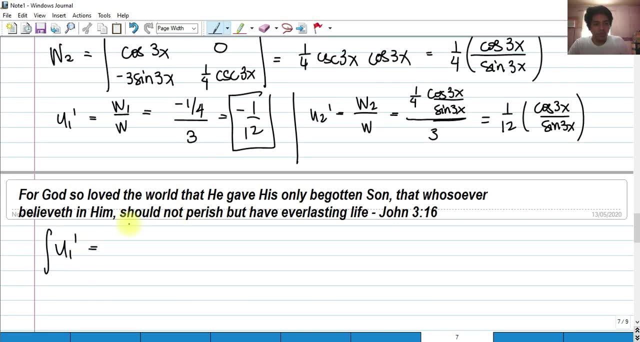 Okay. So again, what are we going to do is to get U sub 1 by integrating this U sub 1 prime, So we have negative 1, 12.. Okay, Since this uses an X, so this should be the X. 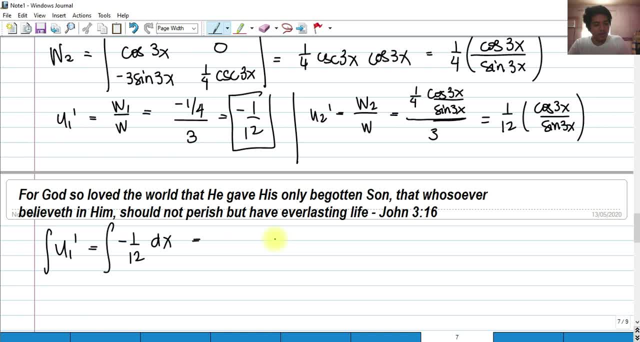 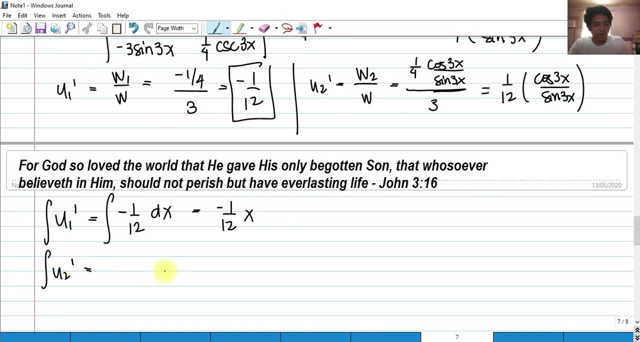 So we have an answer. So we have an answer: to integrate this as negative 1 over 12X. Then we have for U sub 2 prime: Okay, Then we have to integrate 1 over 12, cosine 3X, sine 3X. 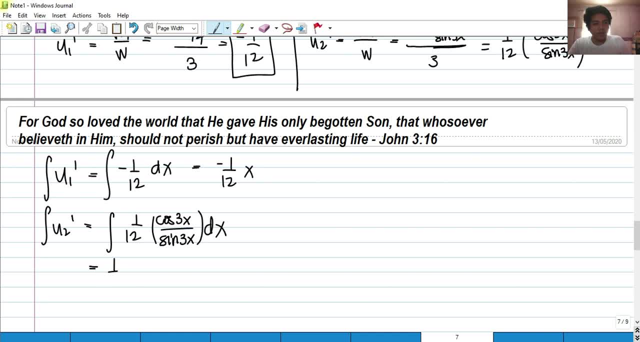 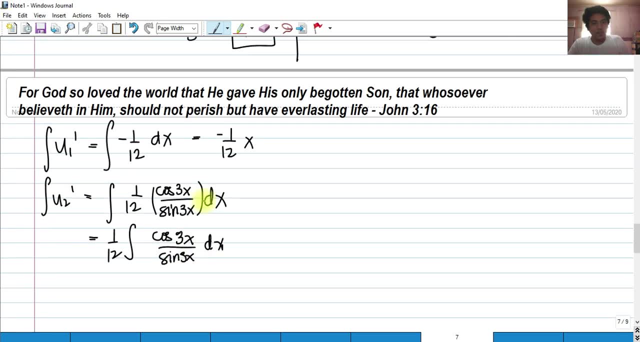 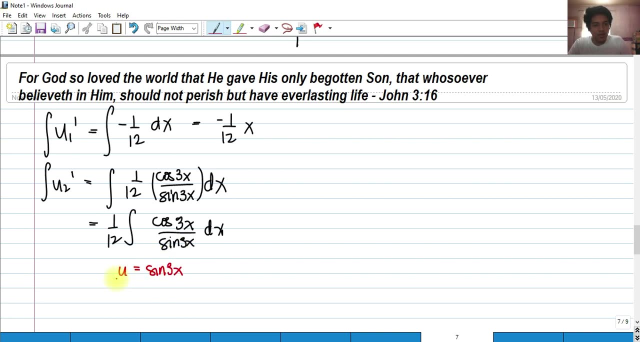 Okay, TX. So we can factor out the constant 1 over 12.. Then we have cosine 3X over sine 3X DX. We can- We can- use U substitution by letting U as sine 3X. Our DU would be 3 cosine 3X. 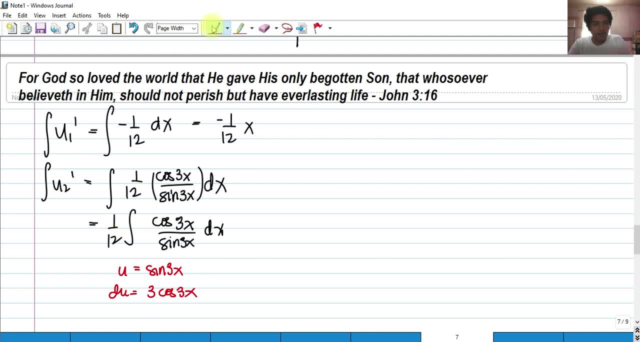 So we don't have any 3 here. So we will be having what We'll be having. We have to offset 3 here. If we offset 3 on the numerator, then on outside of the integral it should be 1. third, 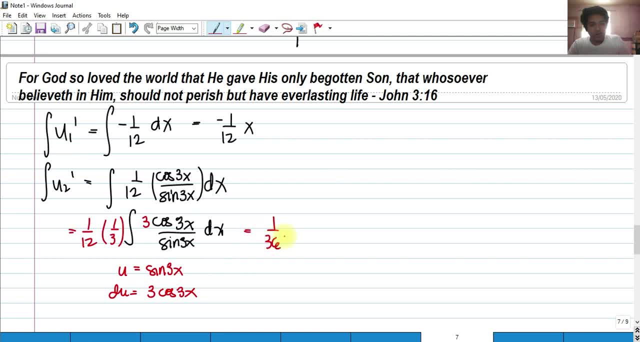 The reciprocal, So that we can proceed With the direct integral of that. So this would become DU over U, And that is 1 over 36 LN of the absolute value of U, Wherein our U is equal to sine 3X. 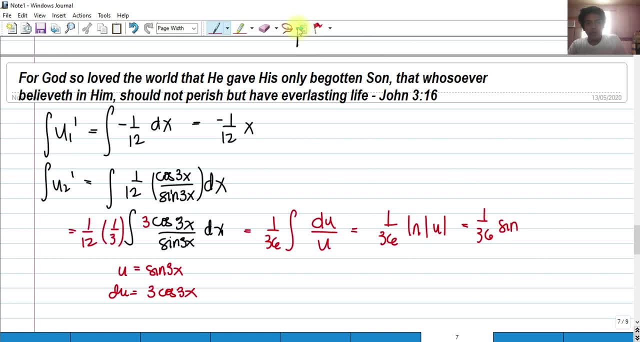 So we have 1 over 36 sine or LN of the absolute value of sine 3X. So we got already the values For U sub 1 and U sub 2.. So we now want to get the Y sub P or the particular solution. 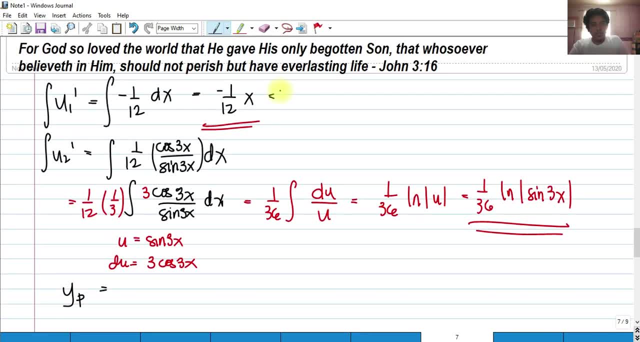 Okay, So we have to replace: This would become the C sub 1.. And this is the C sub 2., Which is also equal. This is to U sub 1. And this is also U sub 2.. This one. 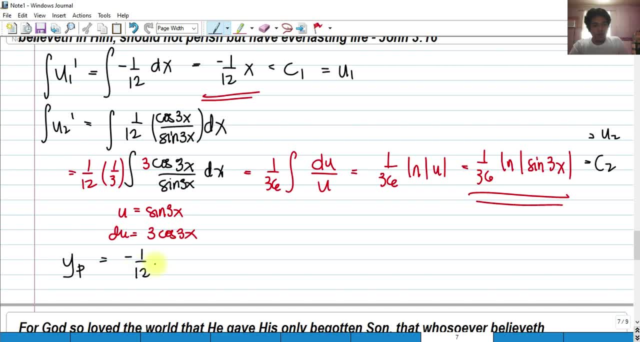 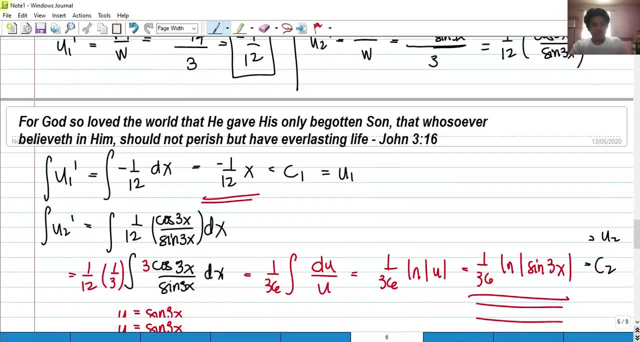 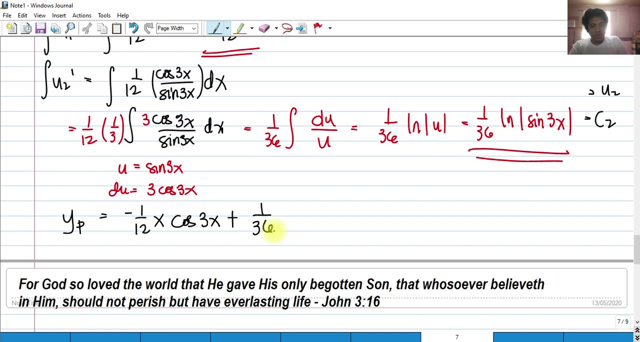 Okay, We simply substitute that We have negative 1 over 12X. Okay, What is our characteristic equation? One Y sub C Cosine 3X. So we have the cosine 3X plus 1 over 36 LN of sine 3X. 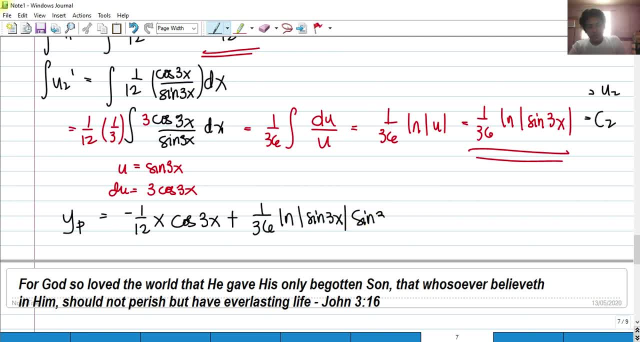 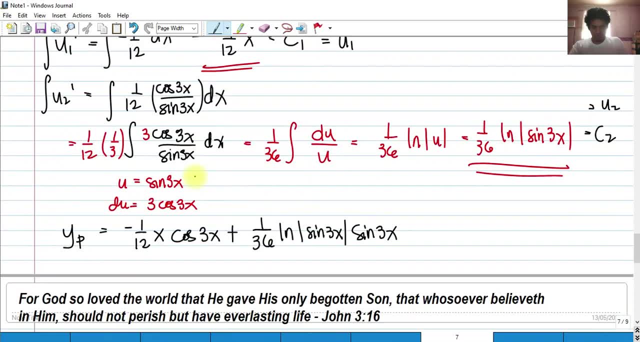 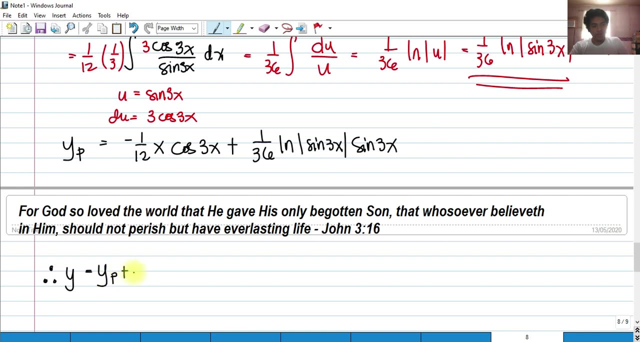 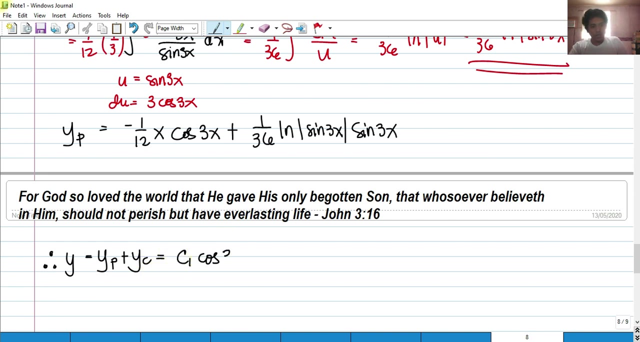 Okay, Sine 3X. If I'm not mistaken, It is sine 3X. Okay, Okay, So our solution would be the combination Of the particular plus the characteristic equation. Let's give first the characteristics. So we have C sub 1 cosine 3X plus C sub 2 sine 3X. 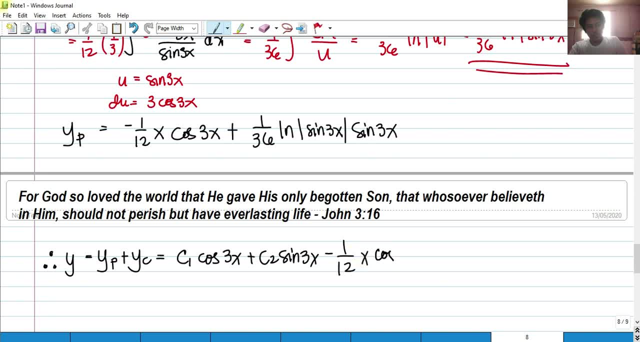 We have minus 1 over 12X, cosine 3X And then plus 1 over 36.. Okay, Okay, Sine 3X, Sine of 3X. Okay, This is multiplied to LN of the absolute value of the sine 3X. 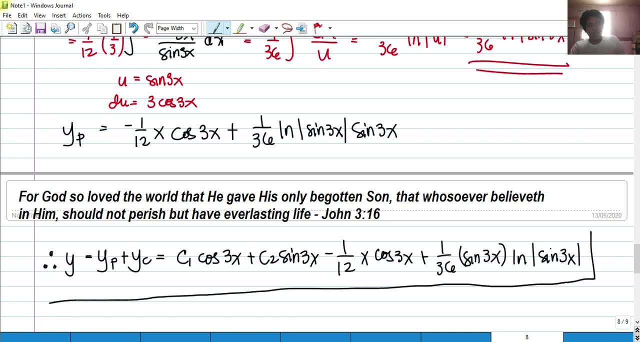 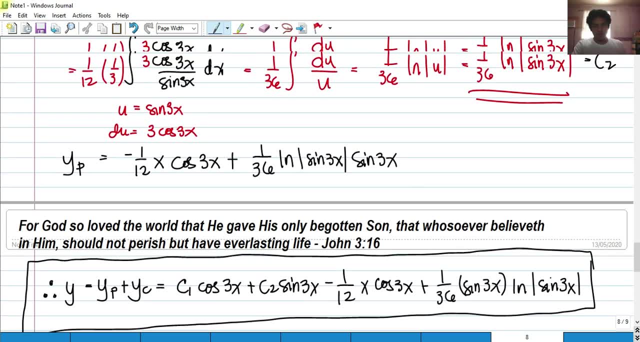 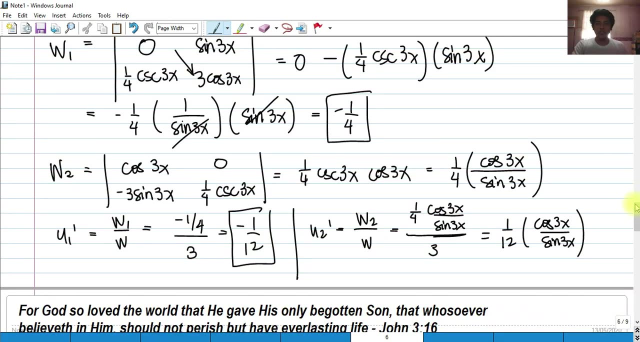 So this is our solution for second order differential equation. On question number two. So, again, if you learn something for this video, for today's video about the variation of parameters, Please don't forget to subscribe to my channel, So or if you are new to my channel. 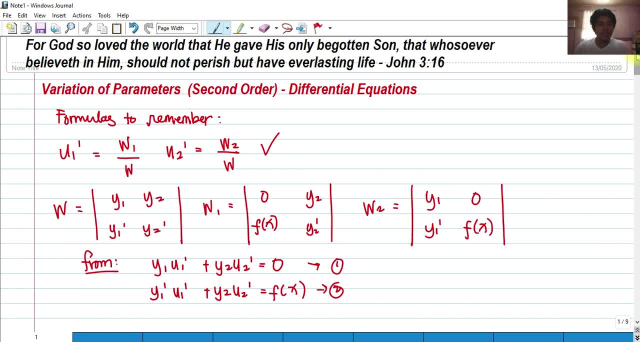 channel, so please don't forget to subscribe to get the latest uploads. all about the math and engineering tutorials. again, this is engineer abba. thank you so much for listening. god bless you.